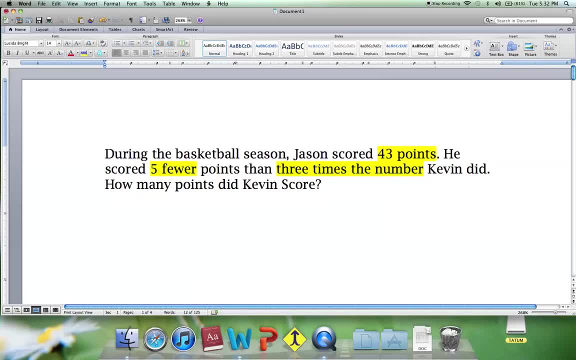 times the number. Okay, so our unknown here is the number of goals scored by Kevin. Okay, so we have 43,. we have 5 fewer and 3 times the number. Okay, so I'm just going to represent n. This is: 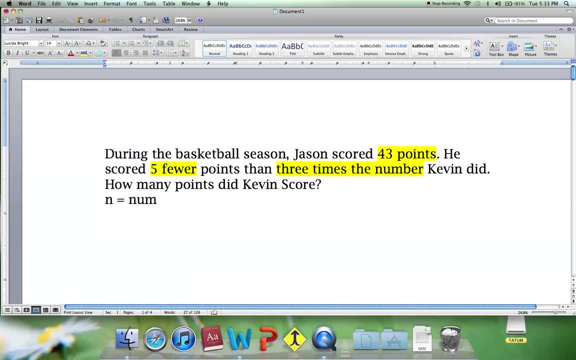 going to be my variable that represents the number of points scored by Kevin, Since I'm using n as my variable to represent the number of points scored by Kevin. if I come back up here to the word problem, I see that I have 3 times the number Kevin did. 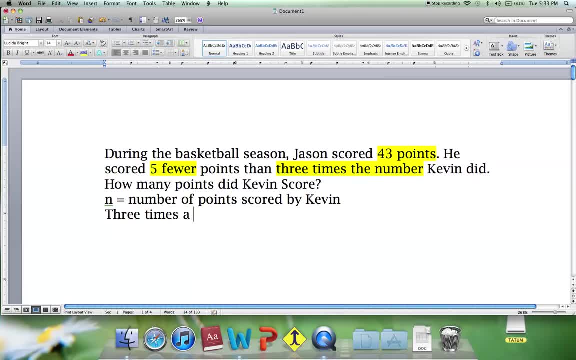 The way we represent 3 times a number is by putting a 3 as our coefficient and then our variable 3n. Okay, So Jason scored 43 points. He scored 5 fewer. This means that whatever 3 times the number Kevin did, Jason scored. 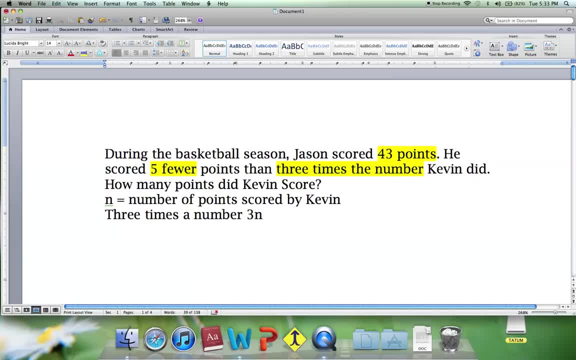 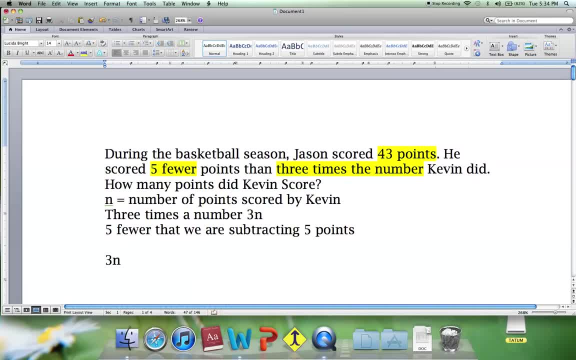 Subtracting 5 points. Okay, So we have 3 times the number Kevin did. minus 5 equals 43.. Now we can solve for how many points Kevin scored, Because now we have a two-step equation. Our first step is going to be to move this minus 5.. 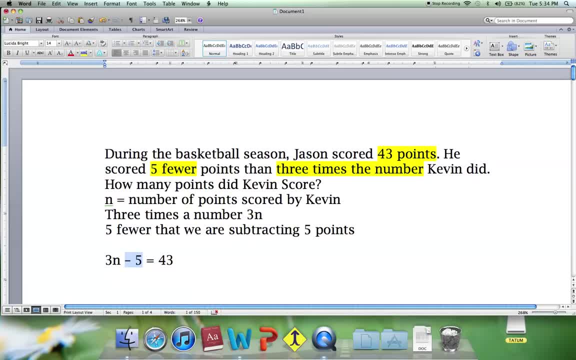 Since it is a minus 5, to cancel it on the left-hand side of my equal sign I'm going to subtract, add it to both sides. So I'm just going to come here and add 5 to both sides. This is going to give me 3n equals 48.. 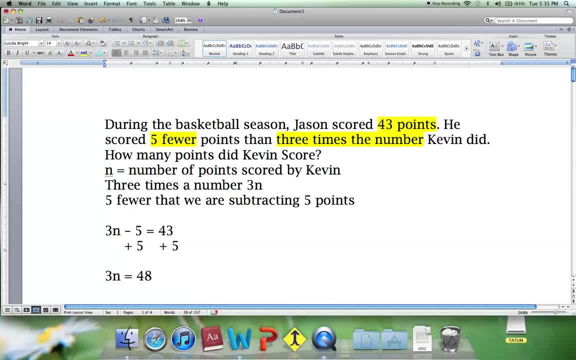 Now I'm ready for my second step in this two-step equation. Notice, I have 3 times the number n. We are multiplying 3 times the variable. The variable is what we want to isolate, Since we have multiplication. the way we isolate that is to divide both sides by the coefficient. 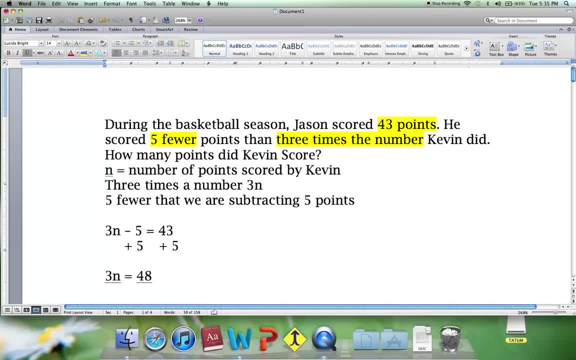 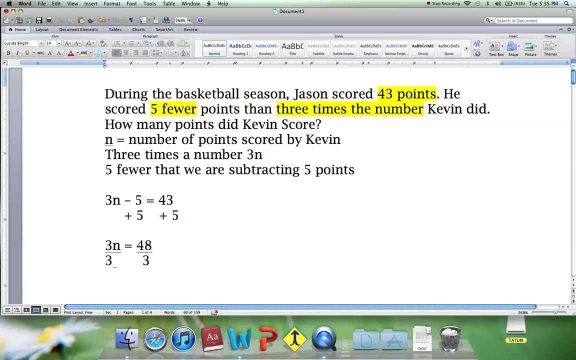 And in this case the coefficient is 3.. So I am going to divide both sides by 3.. If I can get rid of my, So now I am left with n equals 16.. So this means that Kevin scored 16 points. 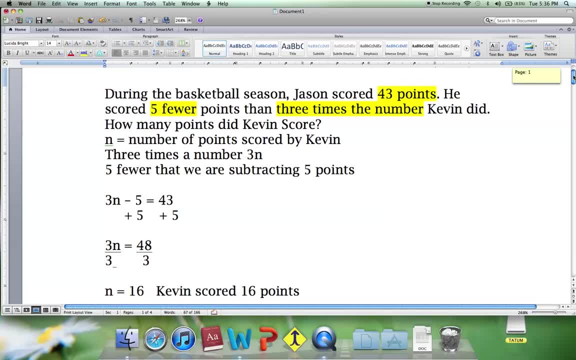 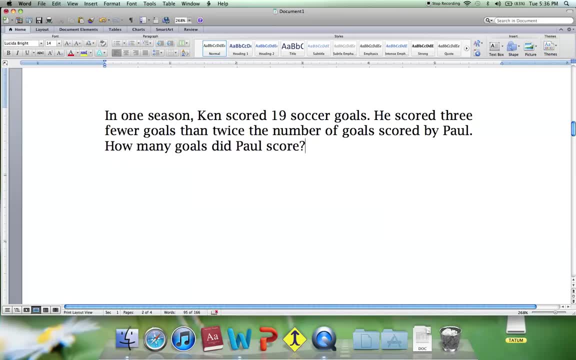 Okay, Alright, let's move on to. Let's move on to the second example. In one season, Ken scored 19 soccer goals. He scored 3 fewer goals than twice the number of goals scored by Paul. How many goals did Paul score? 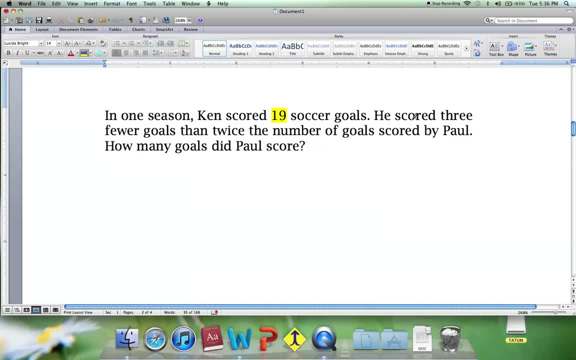 Again, we have our number here, 19,, which is 3 fewer goals. We have 3 fewer goals And, Again, twice the number of goals scored by Paul. Again, we are looking for the number of goals scored by Paul. 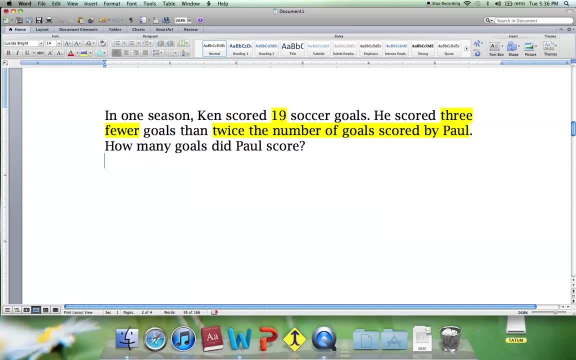 So we have this number twice the number. Well, we'll go ahead and say n is the number of goals scored by Paul. Again, we have twice the number of goals scored by Paul, And to write twice the number, we would write this 2n. 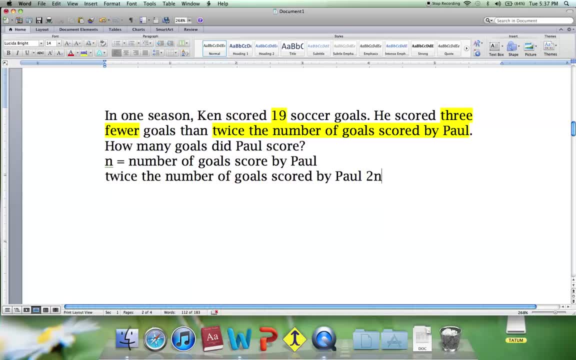 Our coefficient is 2 because we are multiplying n by 2.. And then we have 3 fewer. So Ken scored 3 fewer goals than twice the number of goals scored by Paul. So we have 2n And again 3 fewer means we are subtracting the 3 from the twice the number of goals scored by Paul. 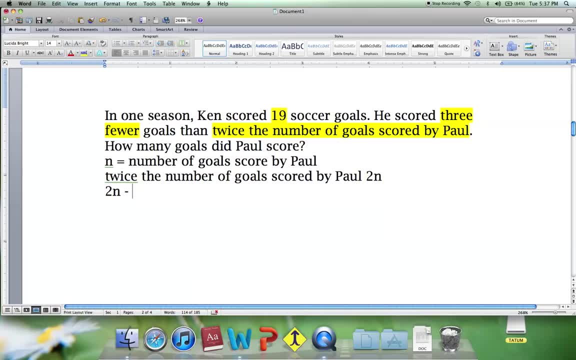 So 2n minus 3 equals 19.. Now we again have a two-step equation. We're going to add 3 to both sides, Because here we can see that we are subtracting 3.. So if we want to get rid of that 3 from the left side of the equal sign, 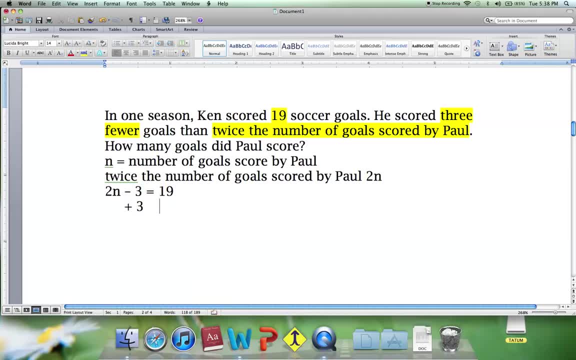 then, what we do to one side, we do to the other. So we're going to add 3 to both sides. This is going to give me 2n equals 22.. And now we're ready for our second step of this two-step equation. 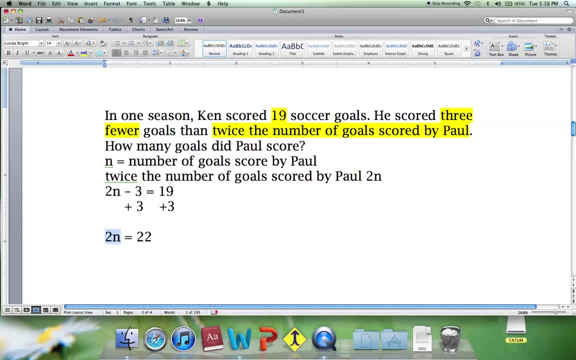 We want to isolate n. Right now the n has a coefficient of 2.. We're multiplying n by 2. So therefore, we want to divide both sides by 2.. Because to cancel out multiplication, we divide. So I'm going to divide both sides by 2.. 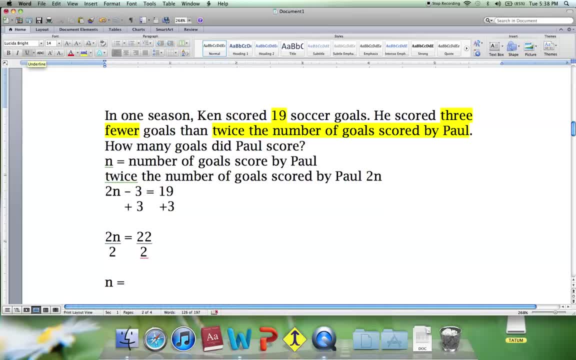 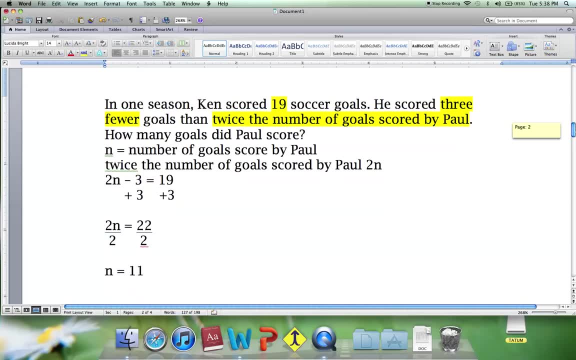 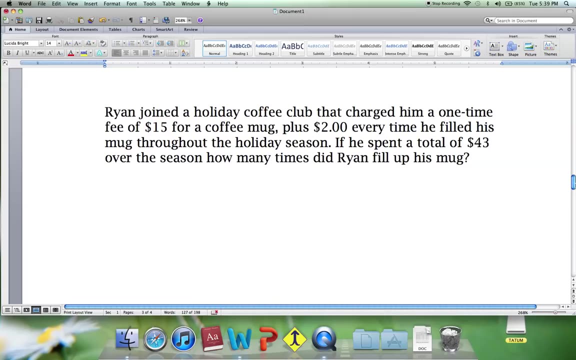 And this is n equals 11.. Alright, example number 3.. Ryan joined a holiday coffee club that charged him a one-time fee of $15 for a coffee mug, plus $2 every time he filled his mug throughout the holiday season. If he spent a total of $43 over the season. 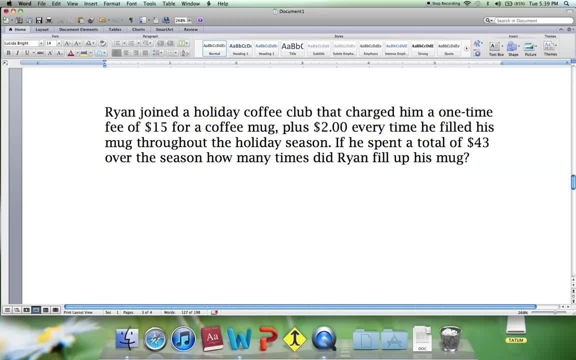 how many times did Ryan fill his mug? So our known numbers here is this constant of 15.. He had to pay the 15 to start with. Okay, he spent a total of $43.. And here is our coefficient. We know that each refill is going to be $2. 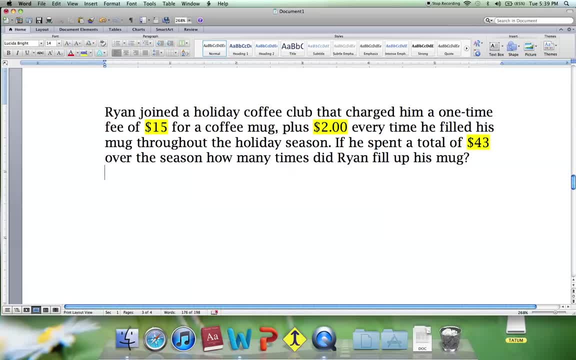 The question is: how many times did he refill? So we're going to use r for the number of times Ryan filled his coffee mug. Okay, So we want to know how many times he filled his coffee mug. That's what we don't know. 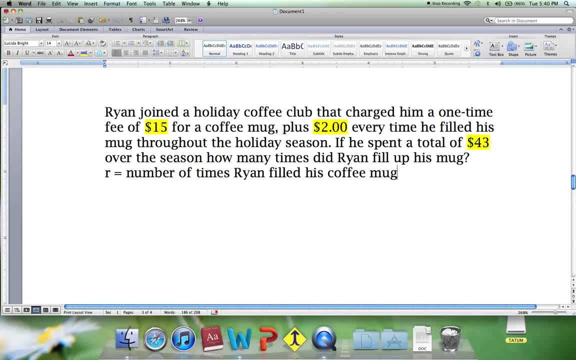 But we do know that every time he fills it he's going to be charged $2. So the way we would represent that is 2r. That is his $2 for every time he fills up his coffee mug. Alright, He spent $15 to get the mug. 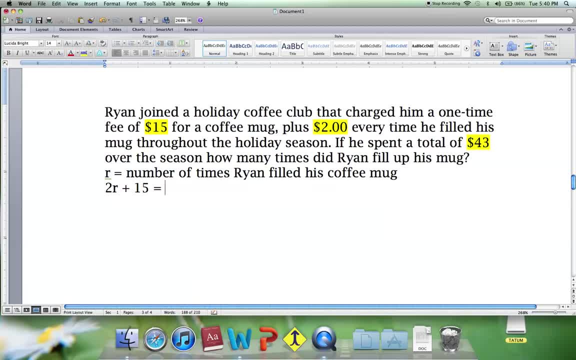 So that's part of his total, because his total was $43.. So of that $43,, 15 of it was to buy the mug. So we want to know the value of r. How many times did Ryan fill his coffee mug? Again, we have a two-step equation. 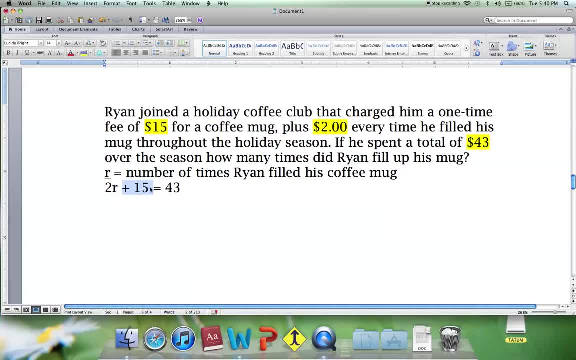 We have a plus 15 with our 2r. Again, we're wanting to isolate our variable, So we're going to move this 15 by subtracting it from both sides. So what we're left with is 2r equals 28.. 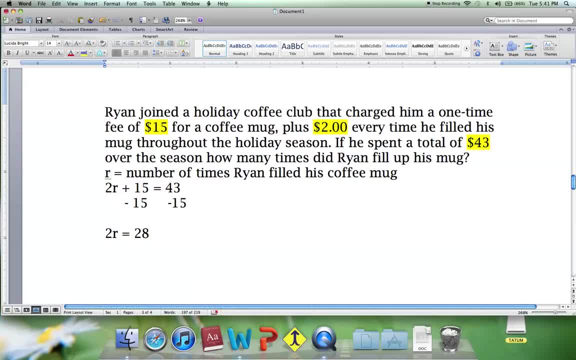 And again, now we're ready for our second step of this two-step equation. We have, 2 multiplying with our number of refills equals 28.. So now I'm going to divide both sides by 2 because, again, to isolate that variable, 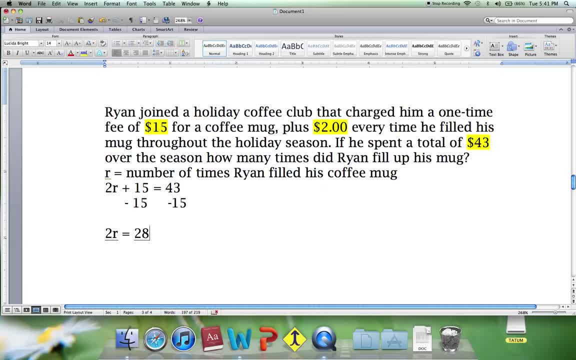 which is currently being multiplied with our coefficient. we're going to divide both sides by that 2 so that we isolate the r. So now we have 28 divided by 2 and we get r equals 14.. Ryan filled his coffee cup 14 times in the holiday season. 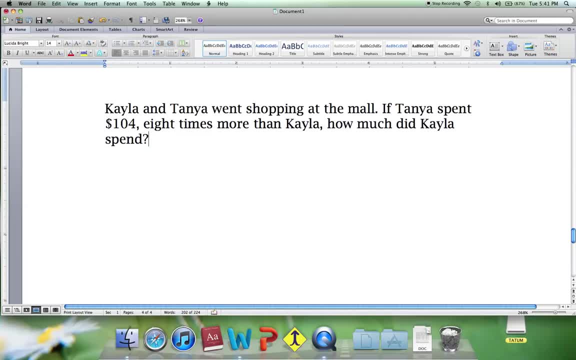 Alright. Final example: Kayla and Tanya went shopping at the mall. If Tanya spent $104,, 8 times more than Kayla, how much did Kayla spend? So we have 8 times more than Kayla being one of the parts of our equation. and $104.. Okay, So we want to know. so we're going to say that x is the amount Kayla spent. Okay Now, if Tanya spent a total of $104 and Kayla spent, or she spent 8 times more than Kayla,